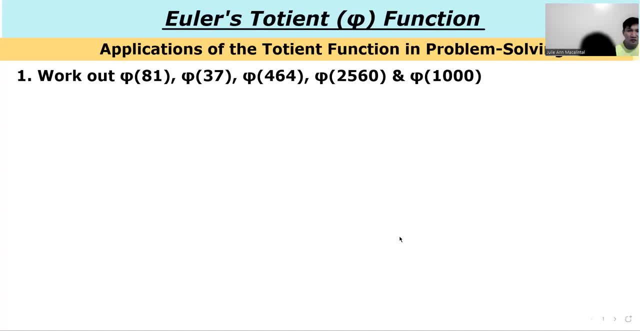 Fraction of 464, Taution Fraction of 2560, and Taution Fraction of 1000.. Let this be A, B, C, D, E, So 4, A, B, C, D, E, A, P of 81.. So 81 is equal to 3 fourths. 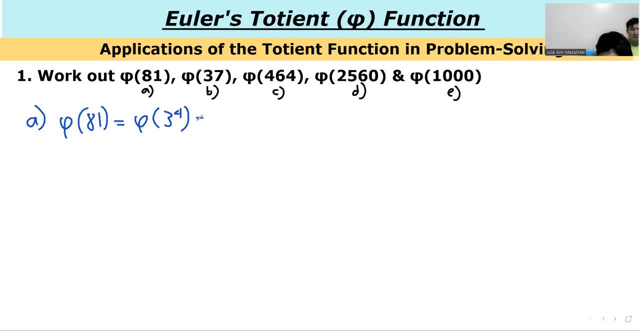 81.. And what's the formula? Can you write it below, And red: Yes, So P of any prime raised to any integer power is equal to that number minus the power before it. So then, 3 to the fourths we can identify. 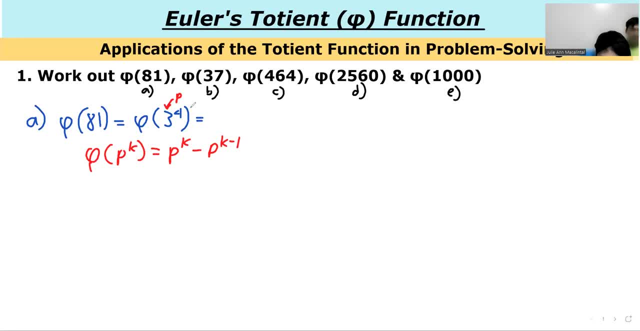 3 as P and then 4 as Q. So P of 3 to the power of 4 is 3 fourths 3 to the power of 4.. Minus 3 Q Or 3 to the 4 minus 1.. 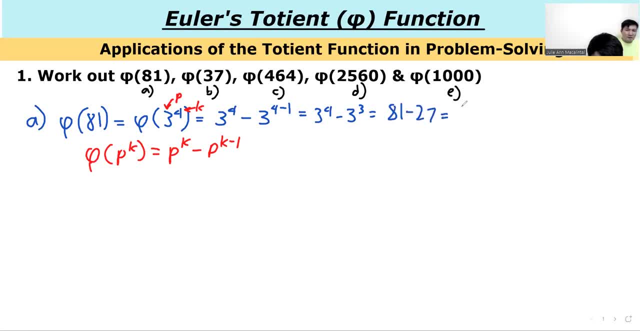 Yes, and that is 51 minus 37, yes. So this is final Boxed. it Nice box. Yes, That's 54. P of 37. So luckily 37 is a prime itself. So formula for: 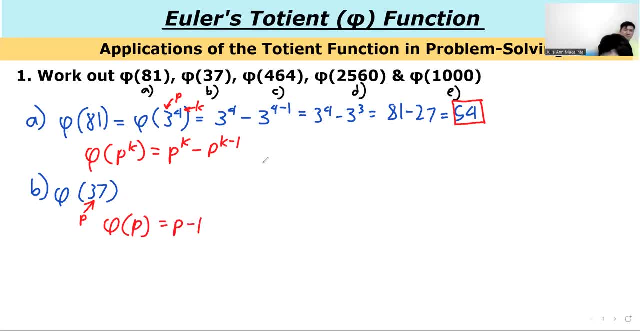 The quotient of any prime is simply P minus 1.. Nice, So easily. this is: 37 minus 1 equals 36.. Yes, Why is it P minus 1? Why is it the minus 1 there? Can you explain to us? 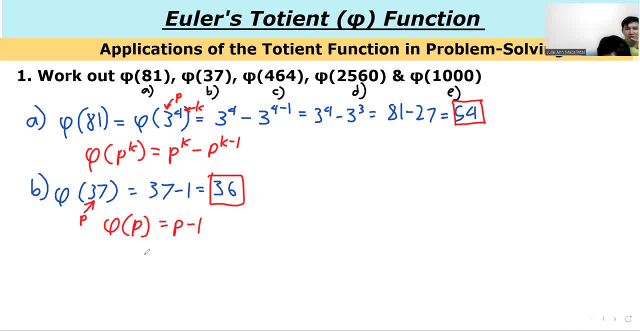 That is 37.. It is 37. Actually, 37 minus 1.. 37. 37.. Oh, I missed the seven. It's the piece. It's the piece on the right. P minus 1 is actually 37,, which is P minus 37 over 37, or P over T. 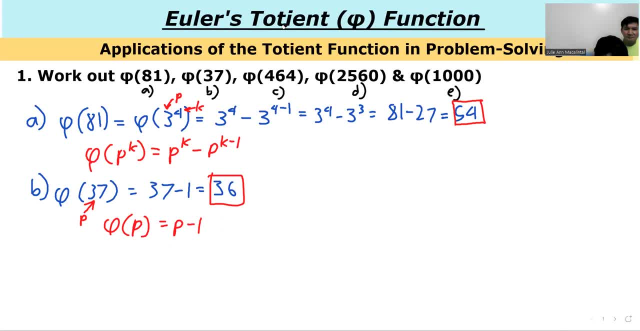 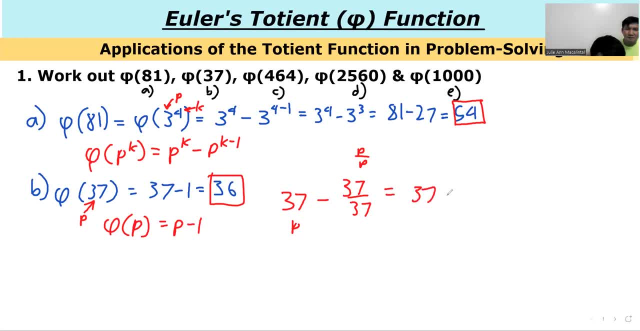 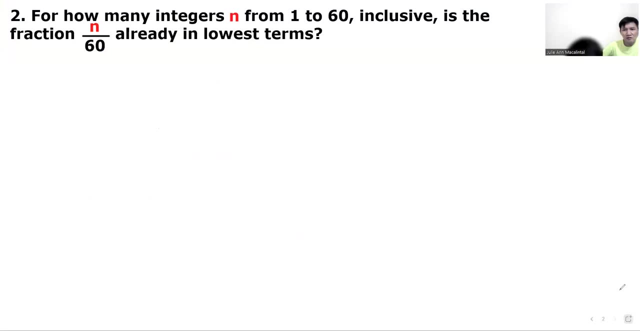 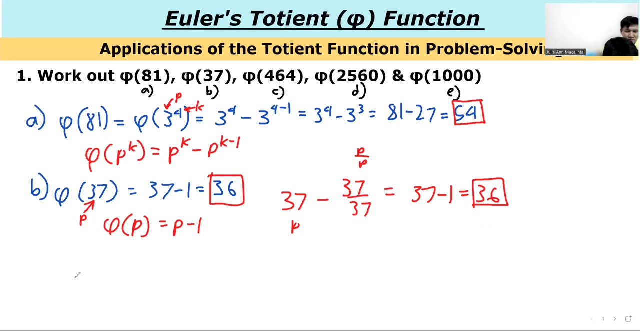 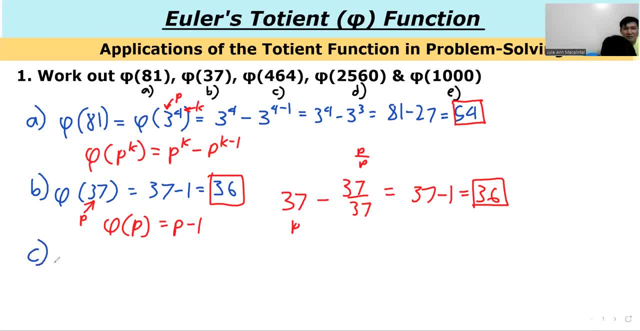 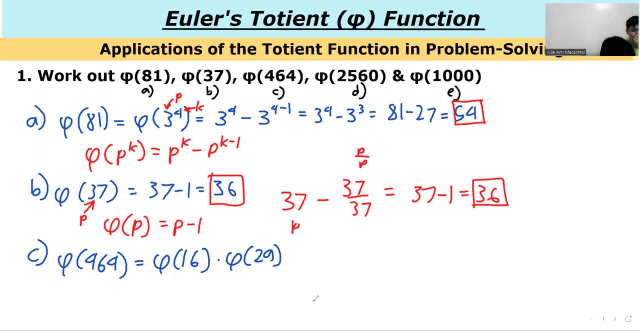 as P16 times P29.. So what formula are we using here? This is a multiplicative a of av equals ki of a times phi of b. Can you explain to us what is in your problem? forces 4,, what is a there and at what's b? So can you explain to us what this in your problem forces? 4, what is a there and what's b, So we can express in in a around, and having the point of 16 times 23V, We can then solve. So just those who are thankfully. 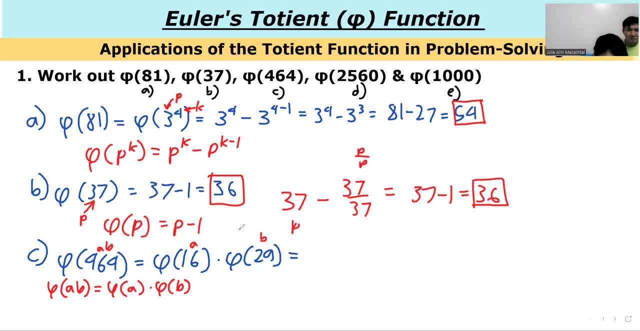 So now we end up with a similar situation to A and B, but there happens to be both of those similar situations. So phi of 16 is the quotient of perfect power of time. So 16 is two to the four. And then the second instance, which is phi of 29.. 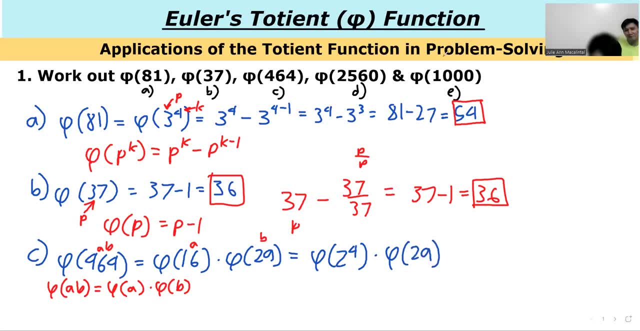 29 is a prime itself. So we're using both formulas, The formula for B. So again I will highlight: So then this is our P, P1,, P2, this is our key. So then that is equal to the first and the second. 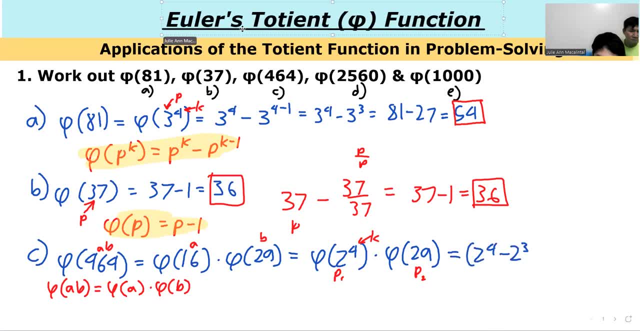 Yes, Okay. So, oops, I'm starting to make minus one, And then eventually this is five: 12 minus 56.. I just let move to the fourth. Oops, 12 minus 56.. Yeah, Um, two to the fourth. 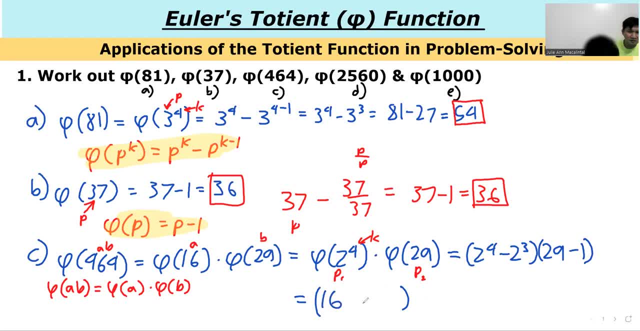 Two to the fourth is 16.. 16 minus eight, Eight and 28.. Eight times 28, 24.. Yeah, Um, nine, Yeah, Three, Three, Two, Yes, Okay. So now we're going to do this. 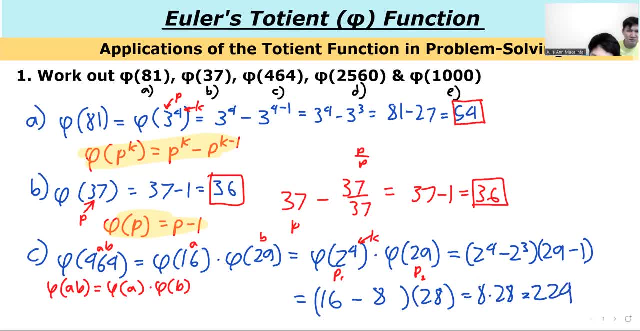 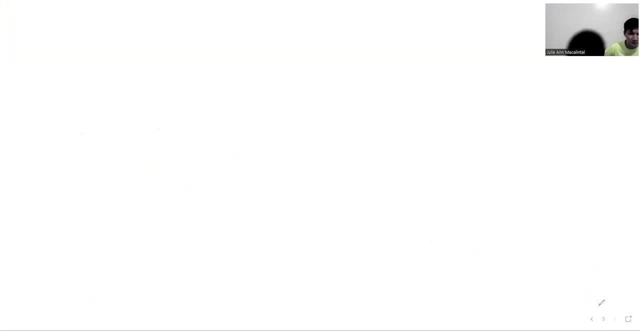 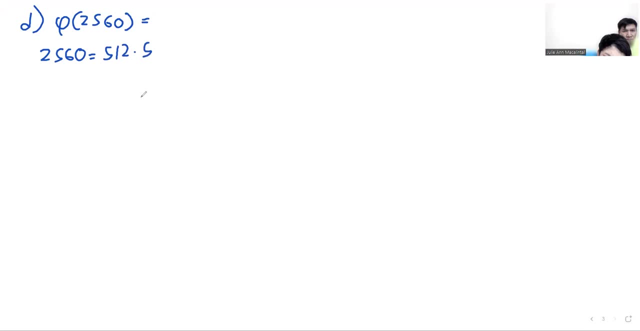 just divide it first: 512 times 5 equals 2 to the 9th times 5,. okay, So this is once again. this is a multiplicative function, So we can just multiply So 5. there is what. 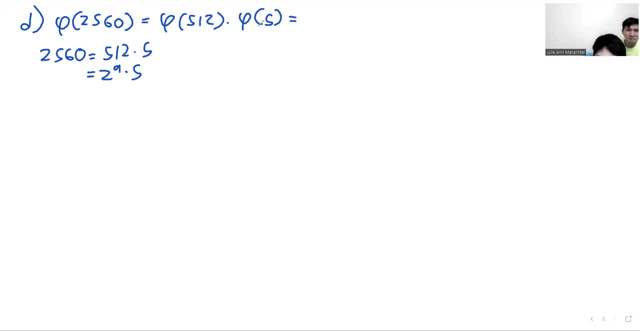 5. there is our prime. 5 is the prime. Yeah, Just be. both of these are already prime, Okay, Prime Nice. So now 512 is a perfect power of 2. Okay, And then 5.. 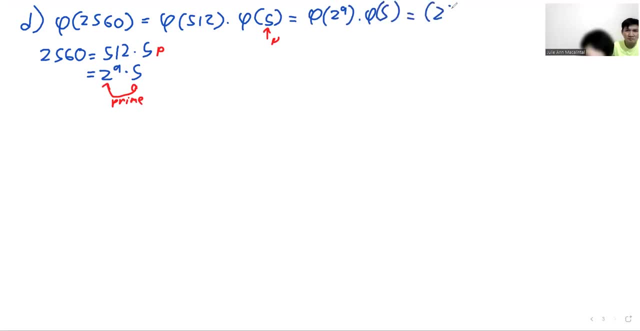 And then we're back to the same situation. Now it is 2 to the ninth minus 2 to the eighth times 5 minus 1.. Okay, It is easier to memorize the powers of two. Yes, We thought that maybe you were learning the binaries, right. 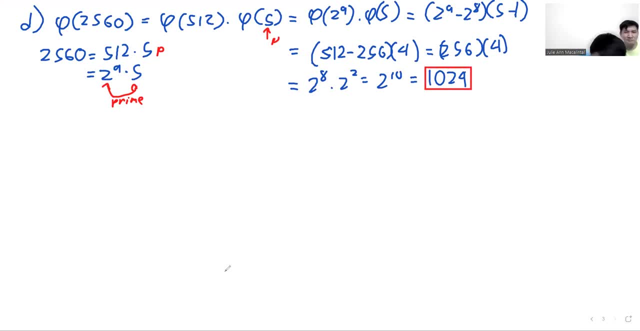 Binaries is also important in many applications, not just the ones related to computers. Actually, I have my own solution For the next number, For the next number. Yes, Can you share with us your own solution? Who are you, My owner? 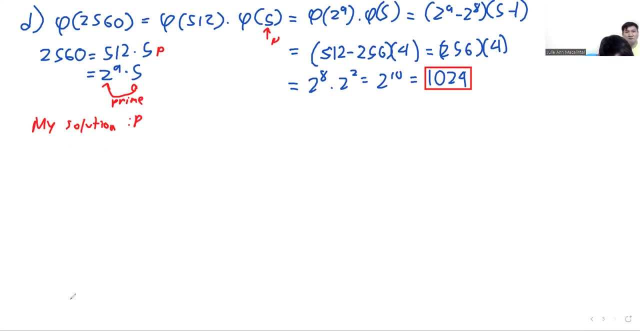 My owner. Okay, Your own. No, Those are all your solutions, but that is your own. The ones you stole from A are all your solutions, but this one is your own, My personal technique. So N equals: It's composed of primes. 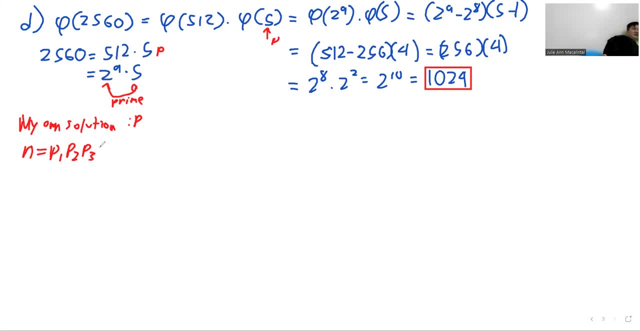 Yes, Any number, Yes, It's prime factorization right. Let N minus N, over its first prime, be Y N Yes. So any number. Private primes: Yes. And'd what you learnt from those Primes. 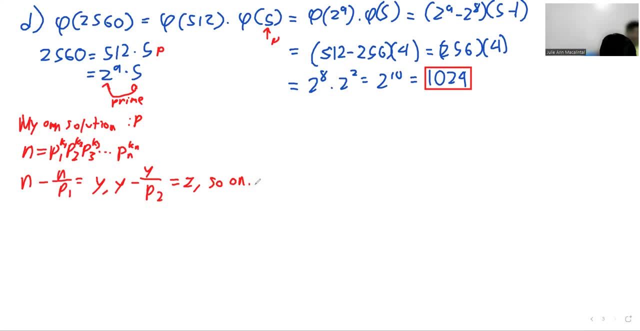 There were no primes, None at all. No, Never again. it just, it just keeps going yes, and then p and q, and this, uh, once once the bn is also converted. so i thought: so q or p is so, once again, these are the price. 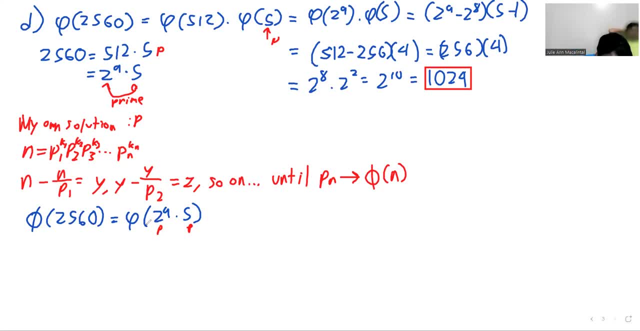 so into the name is what time you're being number one. so now 2560 minus 2560 over two. this can get easier if the prime factorization is rather small. it can get really very, very, it can get very, very big. but, um, if the prime factor, if they doesn't con it, doesn't contain many prime. 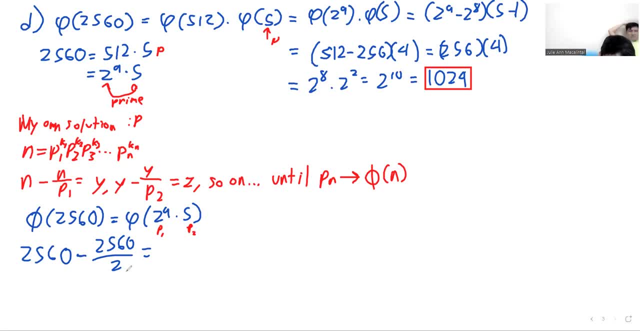 this will be easier than other methods. this is p1. this equals 1 to 80, and then, next step, 1 to 80. it's like it's a reduction minus. the next prime is the denominator. i think prime number two will be the next denominator. yes, if there was a third prime, then 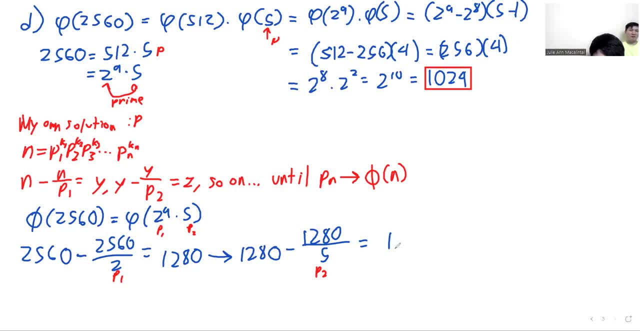 this would keep going, but there are only two primes here, number one in, so the price of decision is 2516. yes, rather magically, i end up with the same solution. it doesn't look like a four. make it like. look like a four, don't make it. 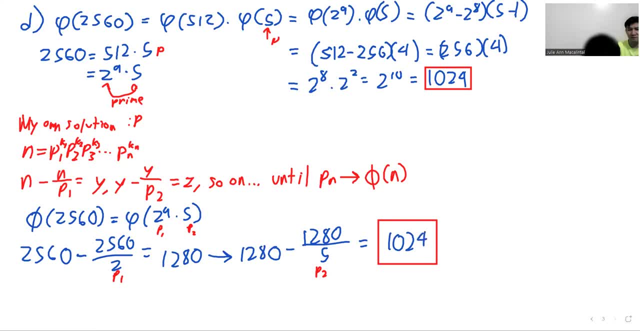 not right. using this one's true. yes, okay, we end up with the same, maybe the same answer for in less steps. but the catch for this, the cashier, is that, uh, if, if, the numbers are very big, and or it has, and, or it has, uh, many, many, many primes in it, it will be rather tedious to do the arithmetic. 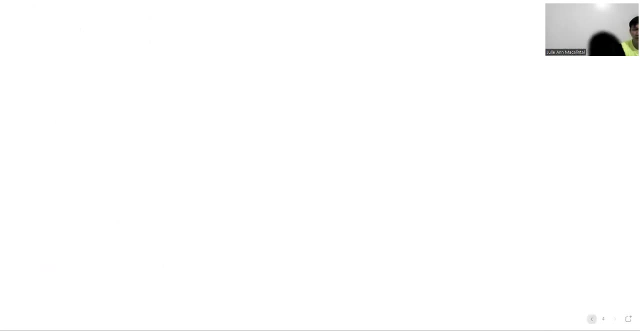 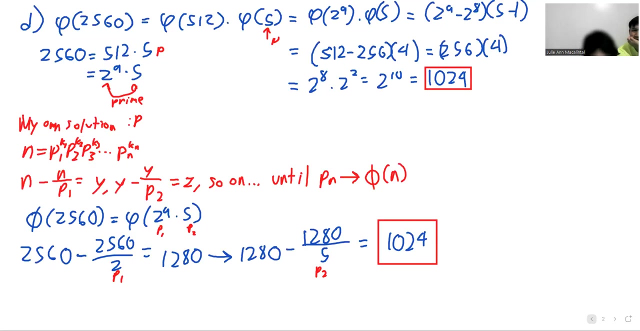 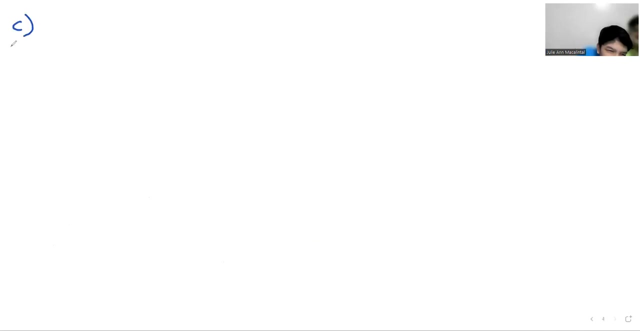 yeah, okay, what about uh trying to do your own uh uh solution on letter, letter c, quotient function, of course, is: where can you try that one if it will work? cc, yes. solution number two, your own solution, po 464, again, breakdown into its prime factorization, which is: 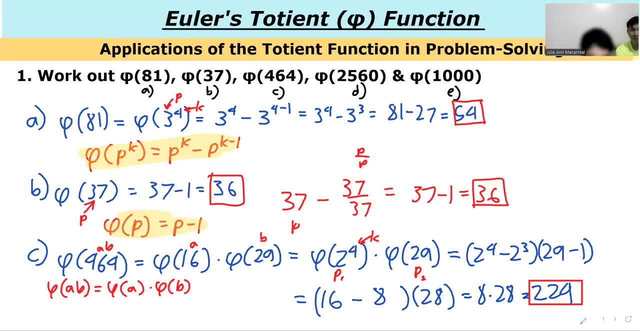 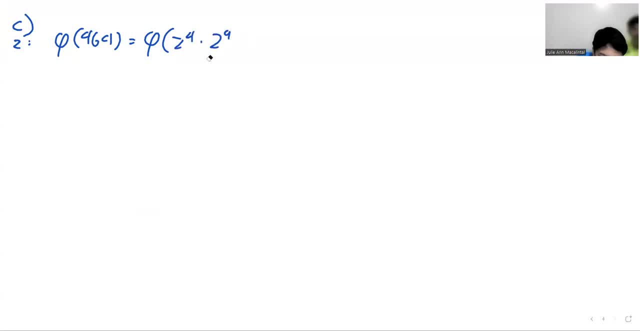 16. 2 to the 4th times 29. 2 to the 4th times 29. thank you 29. 2 to the next. 2 to the 9. no, it's 29. yes, well, it got too small. it looked like an exponent. 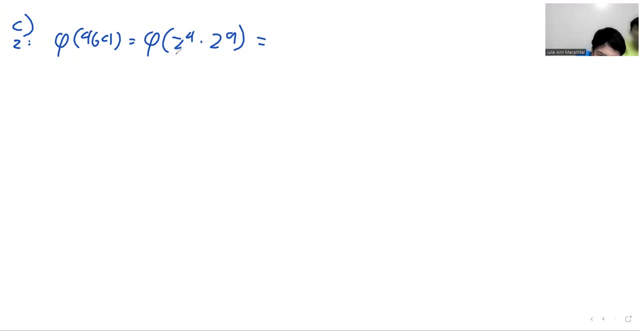 so both of these now are prime number two, primes anyway. so actually there's no. so both of these now are prime number two. so actually there's no. so actually there's no. so actually there's no one thing which I can actually. so actually there's no one thing which I can actually. 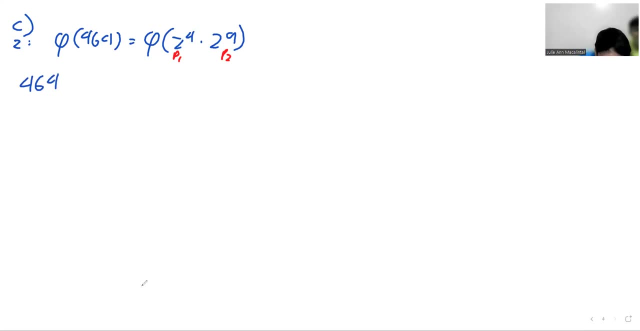 find, you know, Then next step will be. Next step is to take that 232 and then use the next prime. This only works if the primes are in order from least to greatest. Let's see if this is the correct answer. 224, yes. 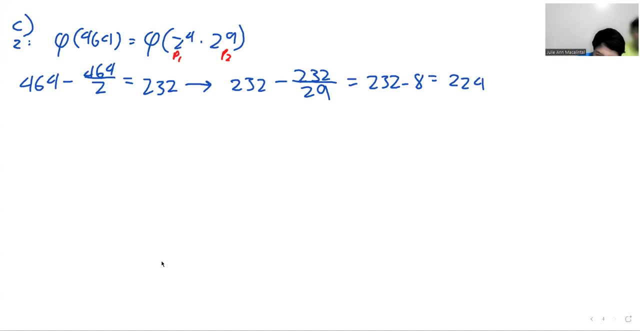 So that's it, Letter E, Letter E. So now The quotient function of 1000.. So Letter E looks. You can expand letter E into 1 million And it will be 1 million. Okay, Okay, Okay. 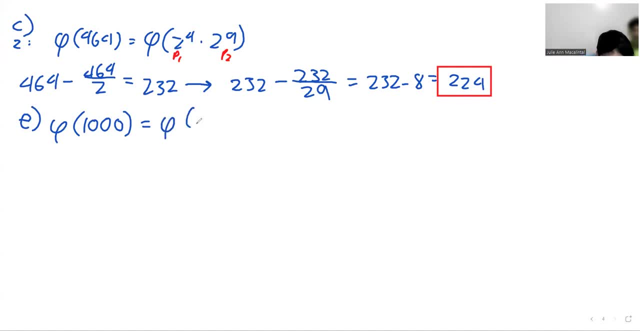 Okay, It would look scary, but it actually is much easier than the others. Yeah, it just looks. It just looks big Power thing, right. So again, break it down into its prime factorization and use the prime factors. 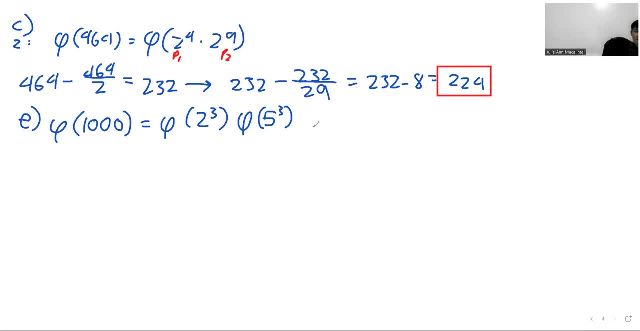 It would be easier if you just break it down. So they are all primes to some power. This is some primes to some power. Yeah, Okay, Okay. So. So 3 cubed minus 2 squared times, 5 cubed minus 5 squared. 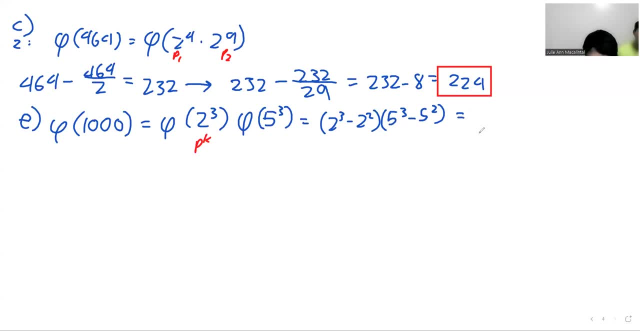 3 cubed minus 5.. Yes, Jock answer: 2 cubed. yes, 8 minus 4 times. I don't have the sound effect noise, so can you try your own uh formula there? uh, algorithm. it's not really a formula unless you, the algorithm is your algorithm. 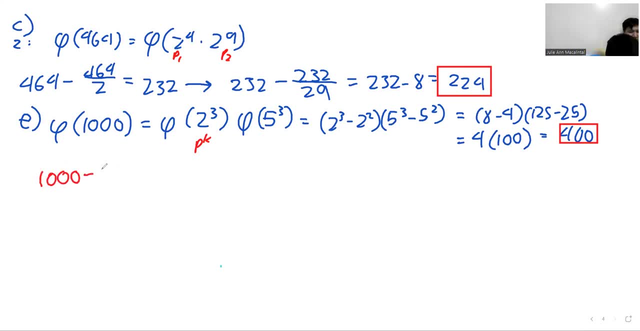 it's not really a formula, because i'll be the last mistaken. five hundred and five, five thousand, five hundred, and then five hundred five hundred over five itself, then that is 400.. so now we can see. we can see why the in the end two is, uh, eventually, a multiple of 100. 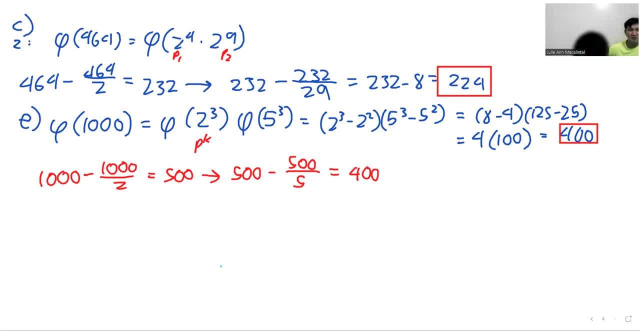 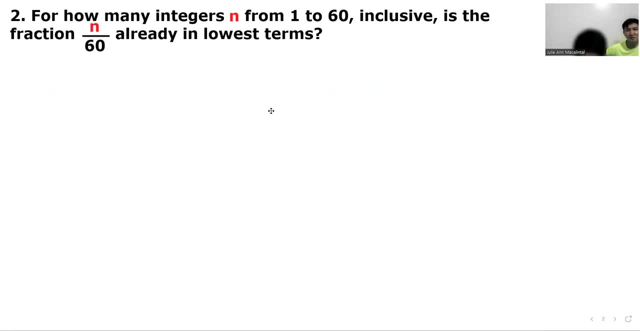 yes, okay, so let's let's go to uh. for how many integers, from 1 to 60 inclusive, is the fraction n over 60 already in the westerns? so first, what are? what do you mean by for those who are trying to learn, for our viewers, who are trying to learn what are functions in the lowest terms? 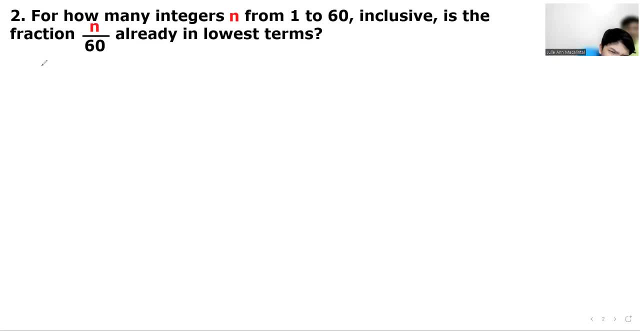 examples. let's say, for example: uh, 9 over 15.. 9 over 15.. let's see 9 over 15.. this fraction is not the lowest terms, because 9 and 15. have a common factor, so that that common factor is three. 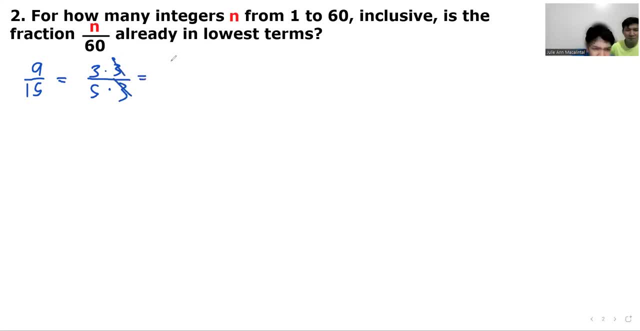 so we can still simplify 9, 15s, do a much more elegant looking. three-fifths, because i can. i cannot take any number, i cannot take another factor from it and then cancel those factors. so essentially the gc, let me. let me, let me add something first here. for example- excuse me, this is not in the lowest terms- because of: 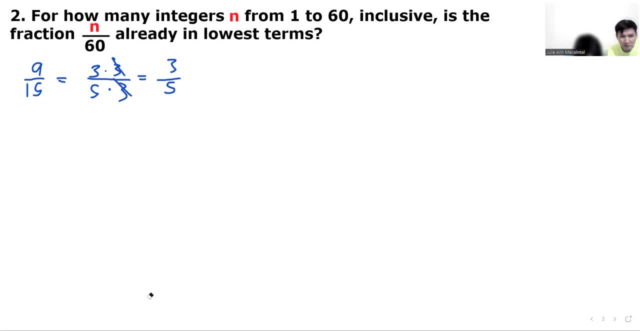 i mean previous one, yes. which one? which one, yes. so here the gcdo of gcd of 9 and 15 is three. so explain to us in. also, in terms of gcd, it means this one, uh, again, we, there's still a difference, not yet in lowest. 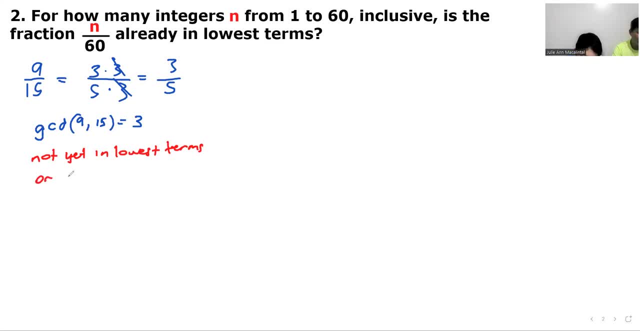 terms, or gcd of three and five. simplest now this. they call this the simplest form. okay, so how about the gcd? uh, what is the gcd of three and five? it's one. it's one meaning. there's a certain history already, sometimes in british english copeland. okay, you like here. well, 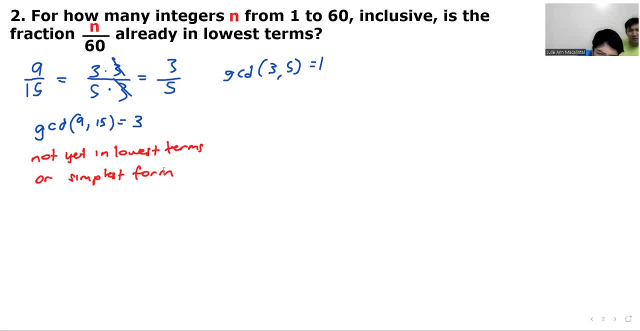 we were trying to learn. 3 and 5 are relatively prime or co-prime. I mean also because there are no more common factors greater than 1 between 5 and 3, so when the GCB of two numbers are greater than 1, it's just 1. 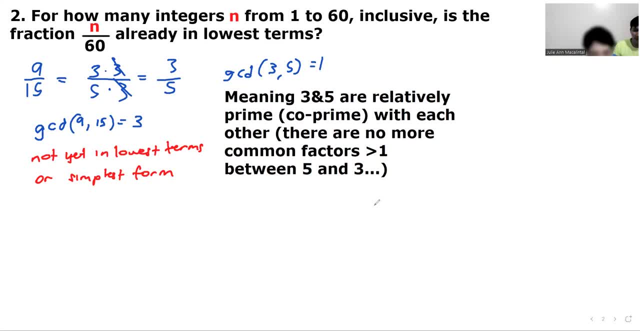 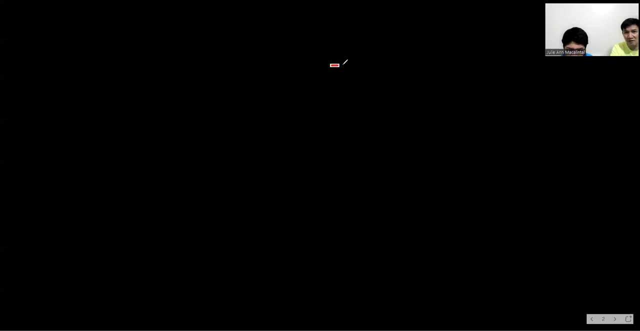 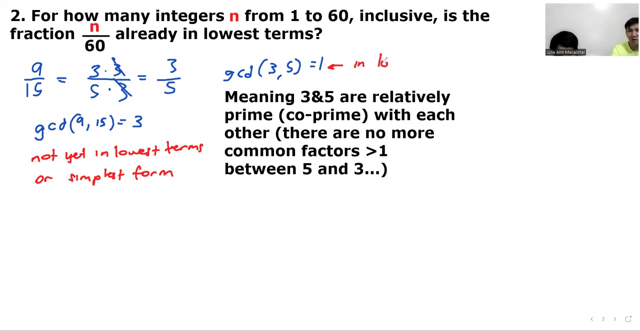 then they are already in their lowest terms. let me just ask for those who are trying to learn: hold on, can you do? you see this already? 1, meaning they are in lowest terms. 4 in simplest form. ok, yes, so we can use this to our advantage. 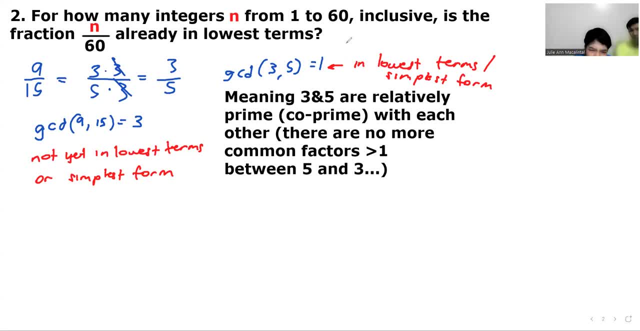 no other common factors or divisors greater than 1. we have successfully converted the problem into mathematics from lowest terms. now we have, we have a function, we can use the lowest function. so we are looking so here in this problem because basically we are looking for what? 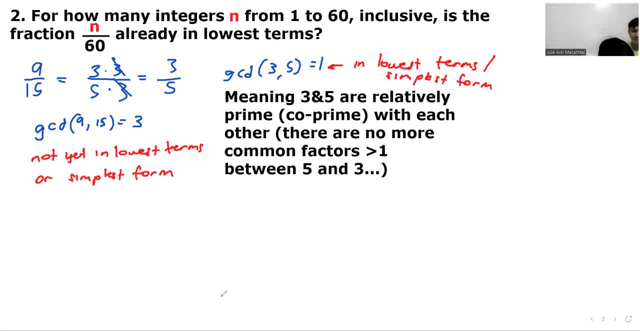 we are looking for the determinant function or 60, so meaning the number, the numbers, let's say the numbers x or number n. you're looking for what? because you want them in lowest terms. so we're looking, basically looking for what the gcd of what this rate. so it's, it would be easier. can you type that? 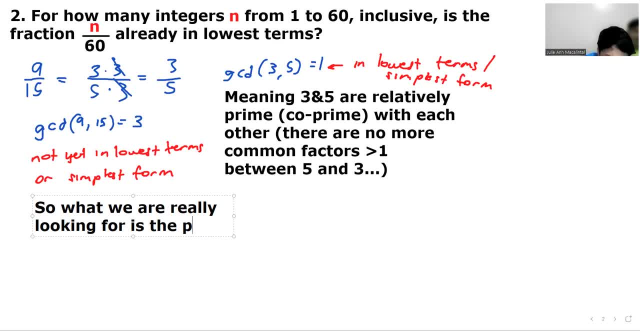 no, no, no, no, no, no, just like the of 60 and 60, and what 60 and what happened. so we are basically looking for what. so we are basically looking for what. we are looking for the numbers. we are looking for the numbers x. i don't see any x there. 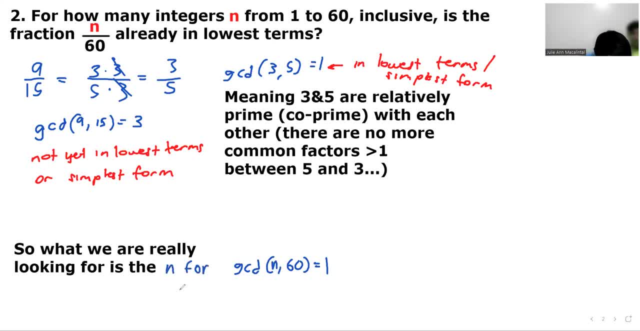 it's the end for which, and so for the end in: uh, when gcd is equal to one meaning when, because, then what? and the gcd is one, it means it means the function is already in lowest terms. so here we go, wait, excuse me. so here we go wait, excuse me. 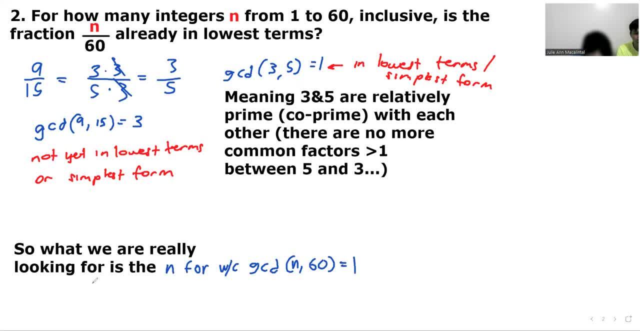 so this is the one i have to press. so here, this is the one i have to press so here. uh, and over 60, right, hold on. and over 60, over 60, so is equal to: is in lowest in. is in lowest in, lowest in, lowest in. 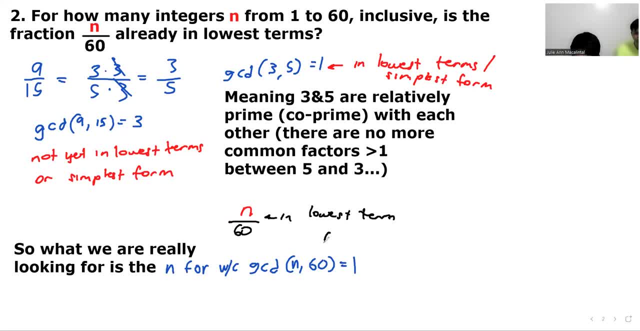 terms, meaning, meaning this one, meaning this one, meaning this one: the gcd of n and 60. the gcd of n and 60. the gcd of n and 60 is equal to, is equal to, is equal to one one one. there are no other common factors. there are no other common factors. 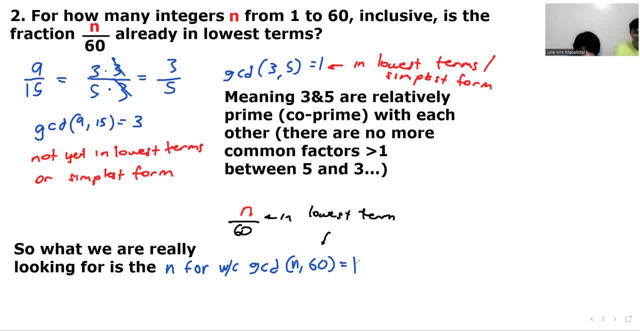 there are no other common factors, more than one between more than one, between more than one, between n and 60. that's basically what you're n and 60. that's basically what you're n and 60. that's basically what you're looking for, looking for. 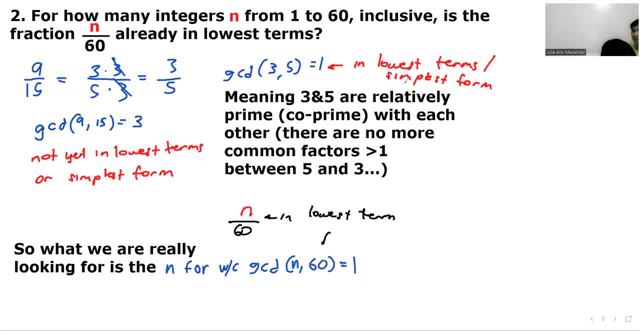 looking for. so, basically, so, basically, so, basically, there, there, there, if, if, if, what's that, what? what's that, what, what's that what you're looking for, what you're looking for, what We're looking for? the totient function of 60.. Yes, we're looking for the totient function of. 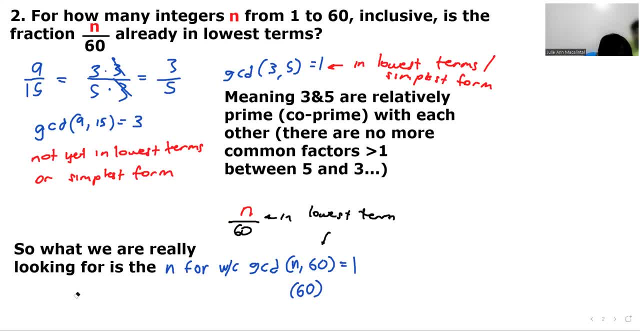 Oh, can you fix that one? It looks like 6.. 6 of 60? The p of 60 or the totient function of 60.. Okay, so now You can use another page, so we don't, And everything doesn't look wrong. 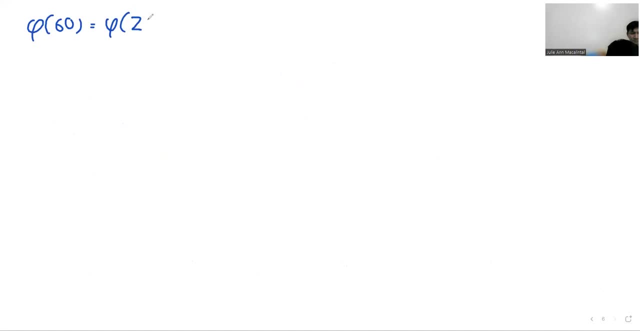 So this is easy. So what formula? Multiplicative function. Let's use the multiplicative function. Yes, multiplicative function of. It's not really the multiplicative function. So The multiplicativity or the multiplicative property of the Euler's totient function. 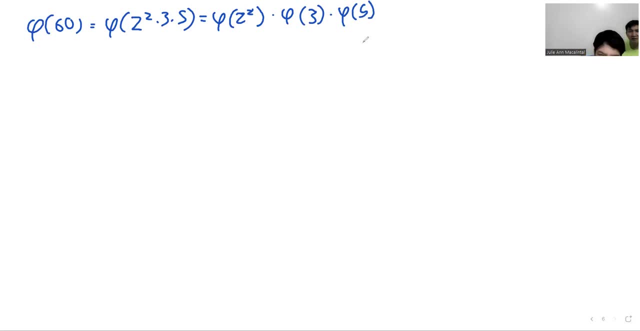 Write up nicely. please Write nicely. What's that? What's that number? Is that 5 or what Do this one once for writing numbers. So applying the formula, The formula she was using before The window, Put down that one. 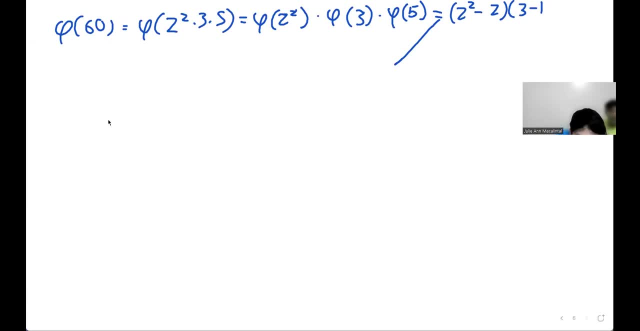 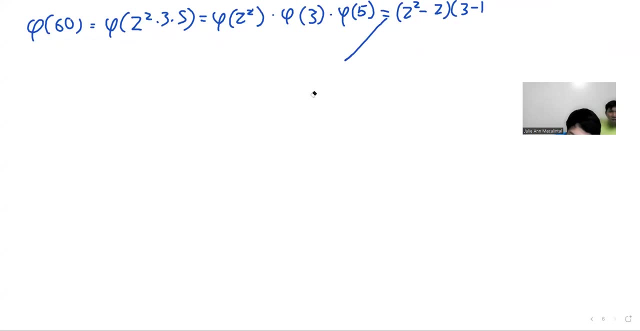 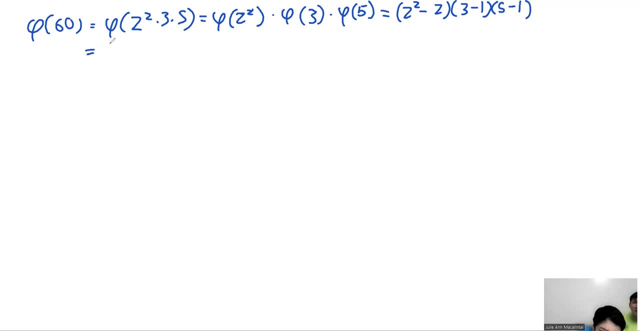 This from type: Yes, Yes, Yes, Just All is written in, All is written in. They can. They can read better just below: Just below it's easier to see: yes, easy, yes, so. or you can use another formula: yes, so that is the alternative, alternative way of. 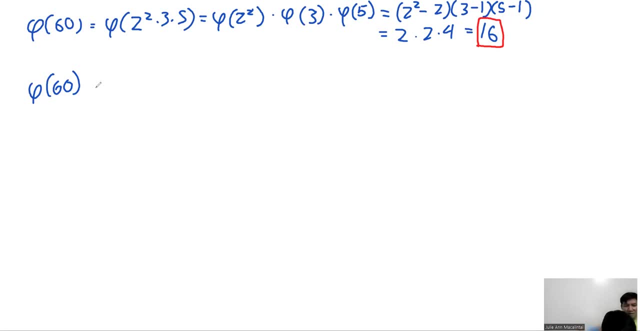 so we will need the prime factorization again. so i'll just put it: careful, write properly, don't rush. can you write more beautifully? so this is two, one of the one of the primes. they become the, they become the denominators. yes, so 40, so 6. 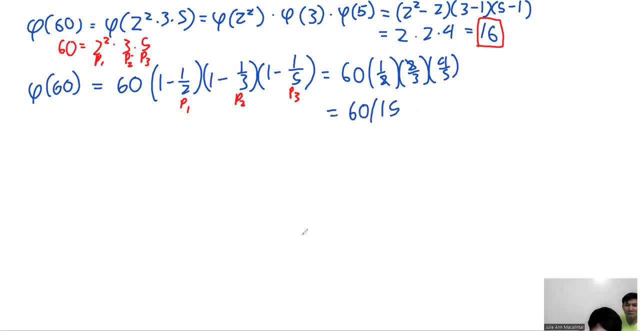 feet or 15 times 4, 60, 3, 4. Oh, you can factor 60 and 5.. Oh yeah, It was 60.. Yes, Can you use your own algorithm here? Yeah, okay, So 60,, so P1.. 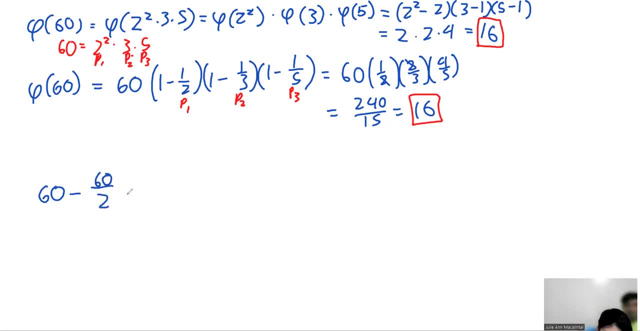 So 60 minus 60 over P1 is 2.. So that equals 30. And then now we will use 30 again, 30 minus 30 over P2, which is 3. So that is 30 minus 10, 20.. 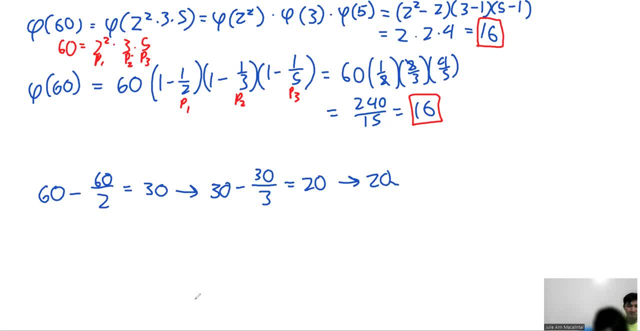 And then next 20.. 20 minus 20 over 5,, which is P3.. So 30 minus 4, 16.. 16 again, 16 again. So let me add something here: What do you mean by 16?? 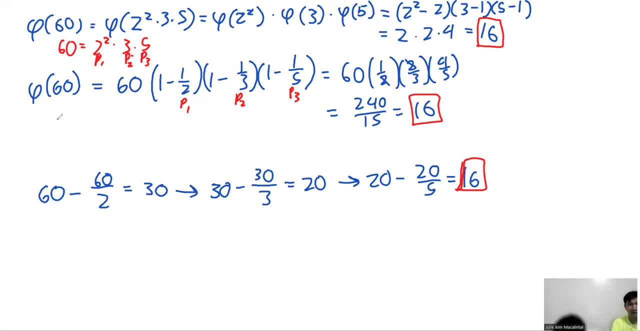 16 is the P of 60, right, It means here's the meaning. I will use a different color. It means there are 16 totatives. Excuse me, Let me move. I cannot move my hand Of 16.. 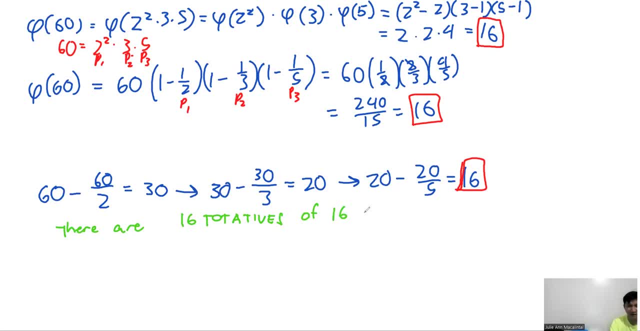 What does 15 totatives of 15 mean? This means that, Can you? I cannot move my hand. There are 16 numbers, from 1 to 16, which are O' or relatively prime with 16.. Okay, I will move this up here. 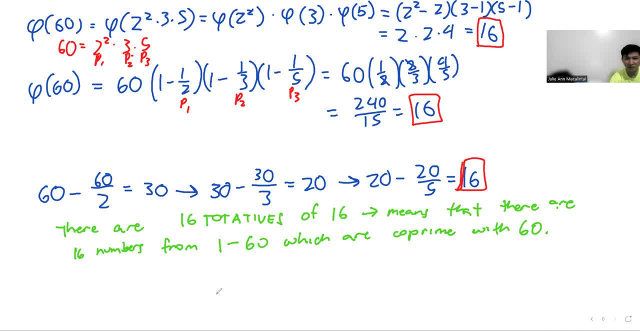 So what are they? So I'll use a different color, Pink. Yes, So they are 1,, 7,, 11,, 13. 4. Those are 4 already, So I'll put a bar, so it's easy. 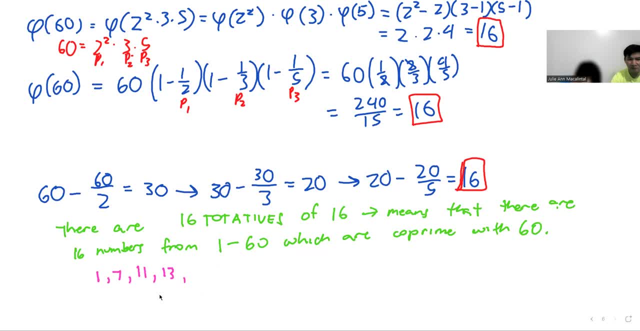 Okay, 2. This is the 19. Okay, So 17,, 19,, 23,, 29,, 31 is also 4' with 16. Meaning they have no common factors aside from 1.. 27,, 41,, 43,, 47,, 49,, 53, and 59. 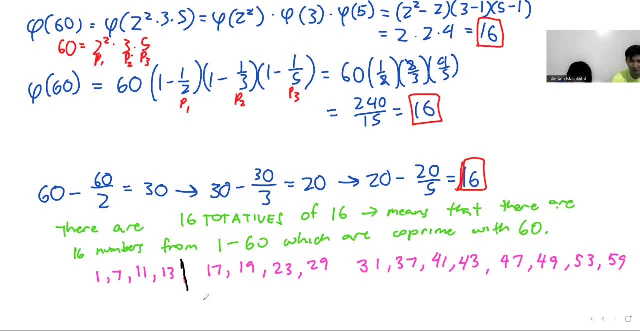 So wait, I will just divide them so it's easier to count by fours. There you go: 4, 8, 12, 16.. There are 16.. All prime numbers which you can use for as your numerator. 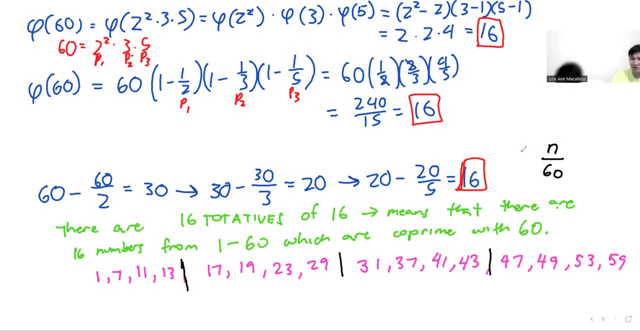 And over 60.. You can either use any of these 16 quotatives here at your numerator And the fraction that you will get will be in lowest terms. So Can you put me to another page please? No, I will just finish explaining this one. 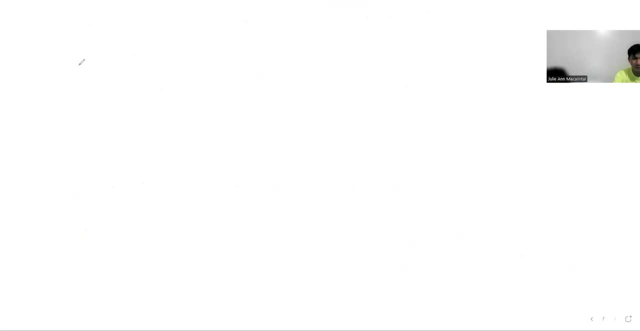 Meaning So I can use an N over 60.. Yes, In lowest terms, When GCD Of N and 60. Is equal to When GCD of N and 1. Equal to 1. Meaning There are no other common factors.